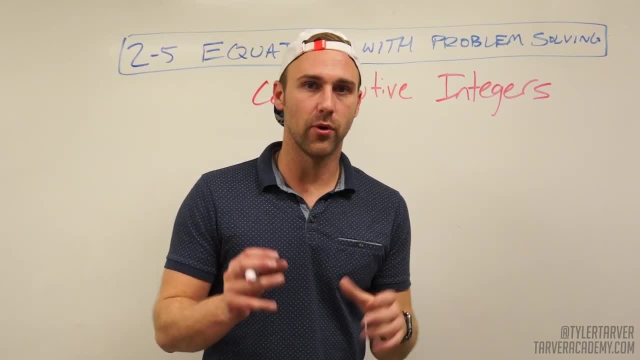 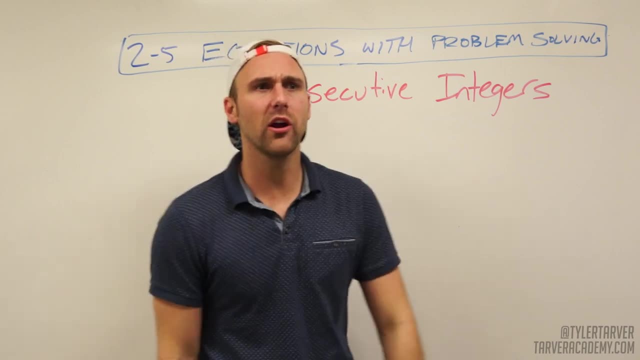 consecutive integers. okay, Like I've said before, with math they're not very creative. They're great with numbers, not creative. And so what they did was they said: well, what are we working with here? Integers, Okay, So like numbers and stuff. Yeah, yeah, Integers, All right. Well, what are? 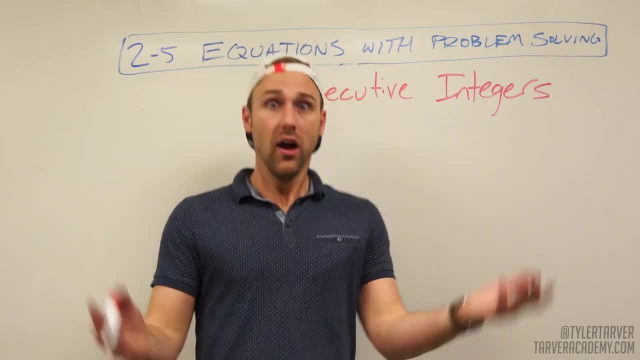 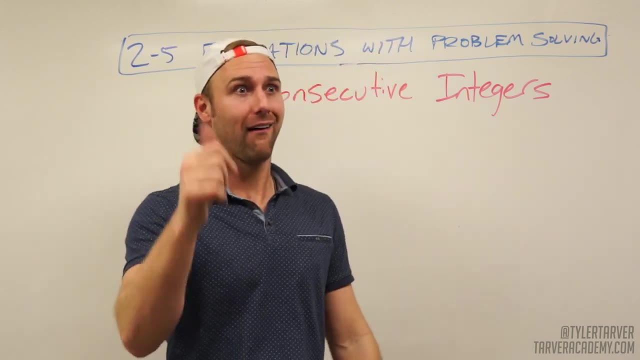 we talking about? We're talking about stuff that's like in a row, So it's like consecutive, right? Let's call them consecutive integers. Oh yeah, Great Math. All right, I don't know why I made that A face. Okay, Consecutive integers: It's talking about numbers that are back to back. 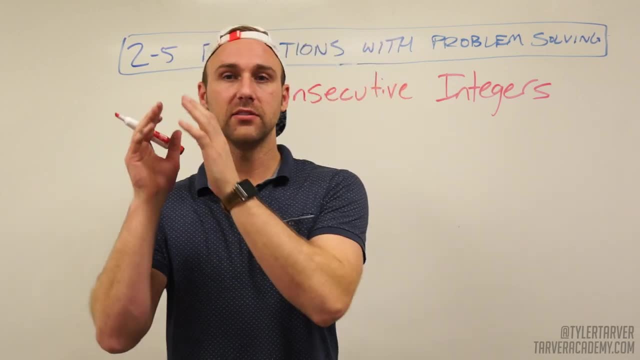 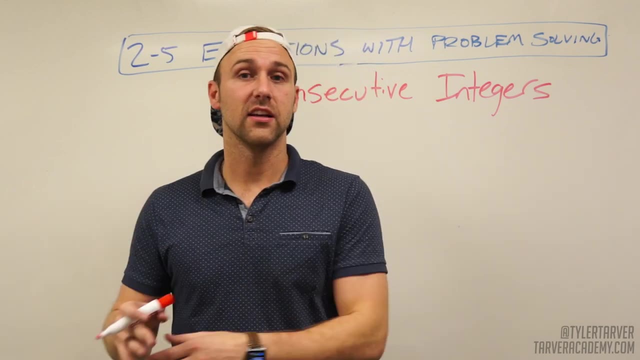 They differ by one number, So like 49 to 50, 71 to 72,, 100 and 101, three and four, 55. And four, five and six, Those are consecutive integers because they go back to back. So when I 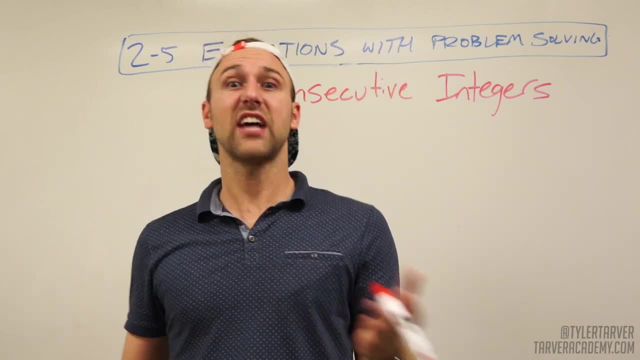 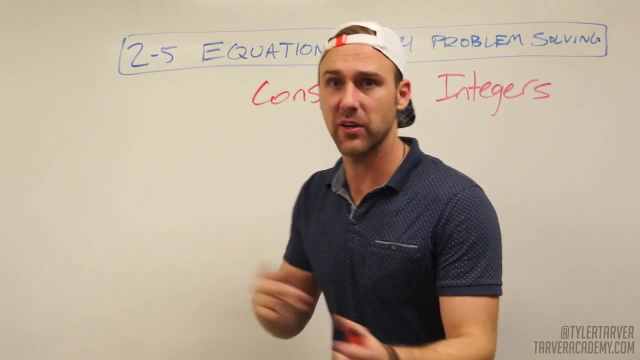 was growing up. the only time I'd ever heard consecutive was like consecutive home runs in baseball. It meant somebody got up there, Boom Home run Score. Next person comes up, Boom Home run. Back to back. Consecutive home runs. It means it's back to back. That's what consecutive 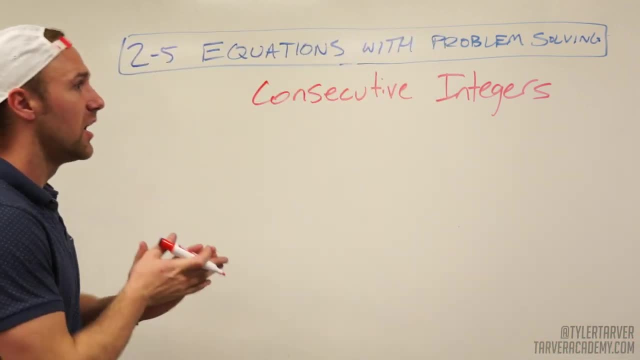 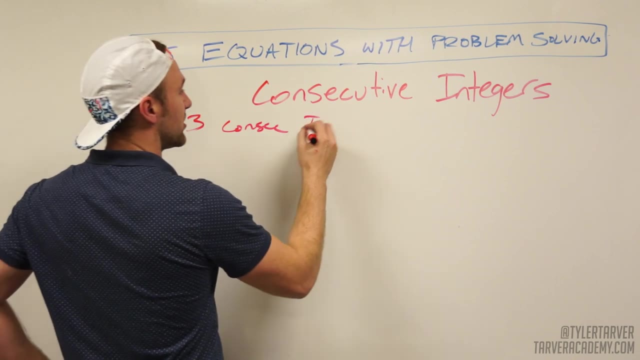 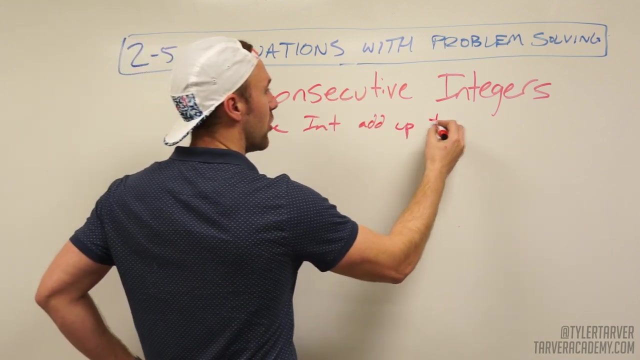 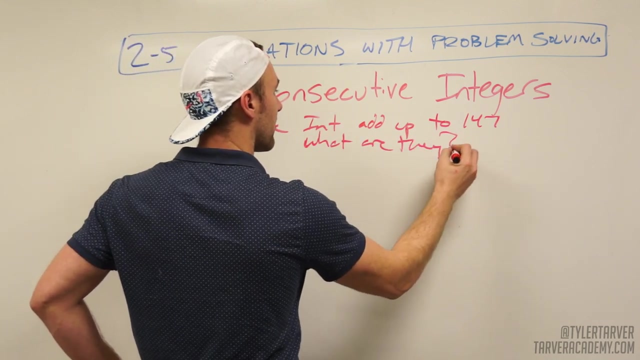 means Okay. So let's look at an equation. Let's say three consecutive integers add up- or the sum of three consecutive integers is the fancy way to say it- to 147.. What are they? A lot of people, a lot of people will just like: guess and check Like. 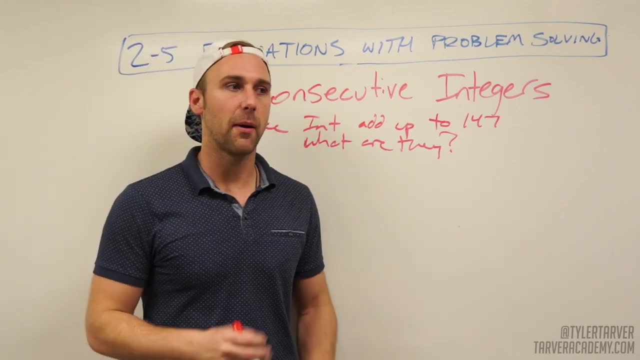 they'll start typing. If they're taking a test, they'll just type of stuff in their calculator. I'm going to show you the equation way to figure it out, but also tell you if you are going to guess and check. say, like worst case scenario, you forget everything. 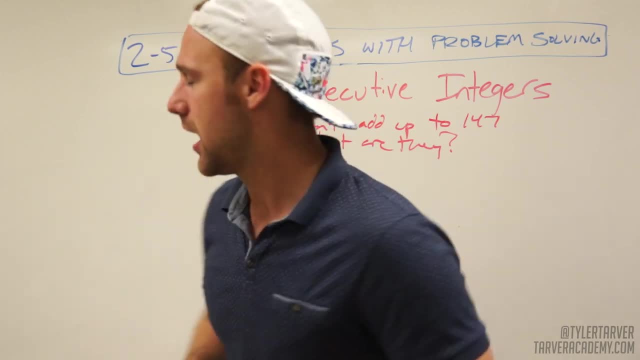 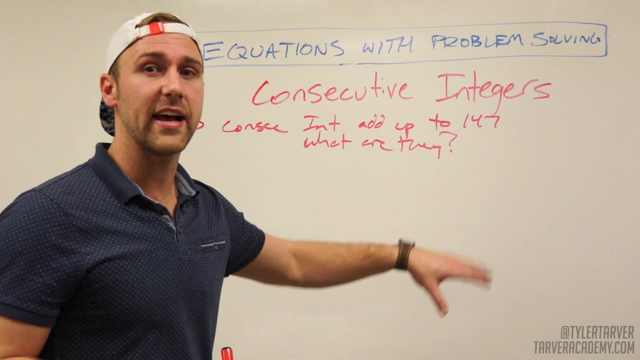 I just taught you which you shouldn't, because I'm going to teach it as well as I can And remember everything I say. Did I ever mention that? Just remember everything. I ever say So whenever you're doing this. if you are going to guess, think: okay, you've got three numbers. 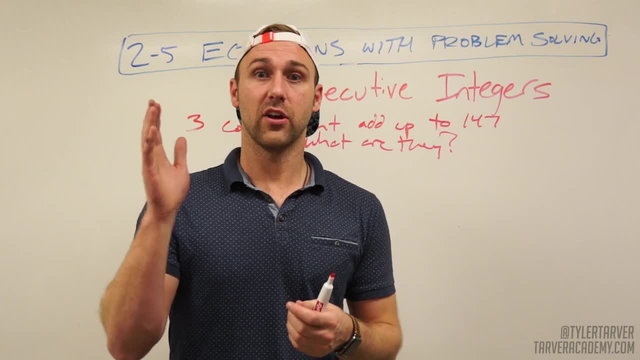 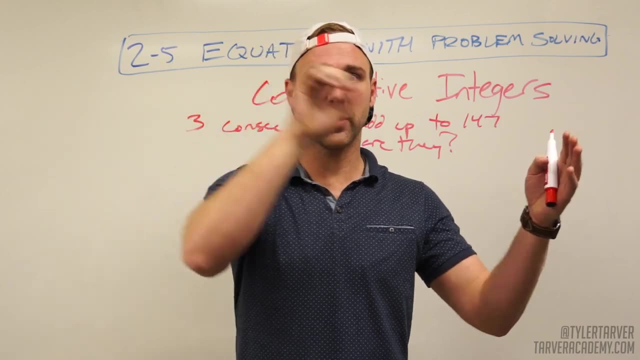 They're going to add up to around 147, which is close to like 150. And they're going to be back to back to back. Okay, If you've got around 150, split that into three chunks, because if numbers are off by like one, they're pretty close. So you're like 50,, 50, 50.. That's 150, right. 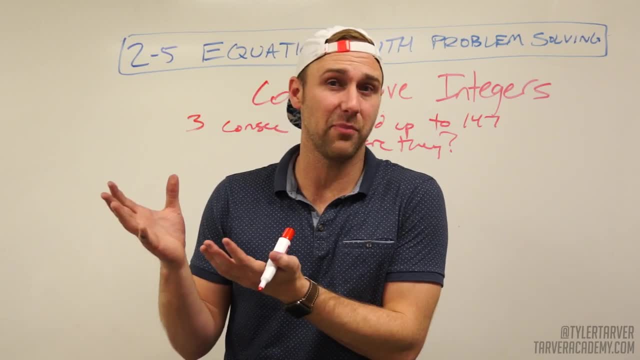 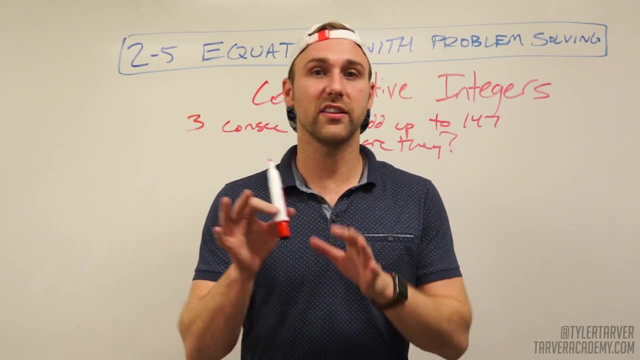 So you know that your three numbers are going to be close to 50, give or take probably five. That's my guess. All right, Cause you know they got to add up to that, but they differ just a little bit. So I guess they're probably somewhere around like the 48,, 49,, 51, 52, 53 range, But I'm 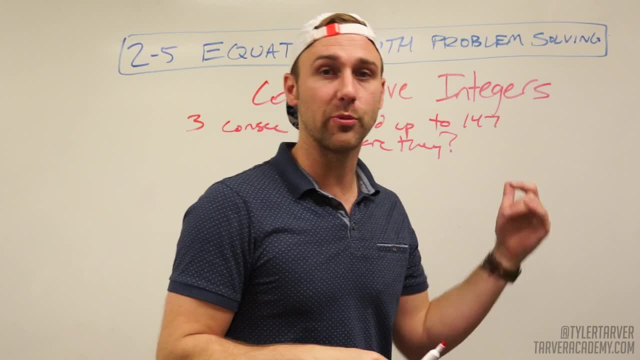 going to show you how to work the problem: legit style. So you can write it out, So you can open response. You can write it out: look really smart, make your teacher look good, Then your school look awesome. They're going to celebrate and you're going to win a million dollars. That's. 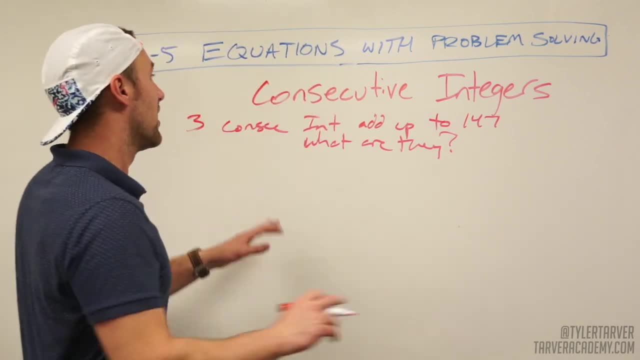 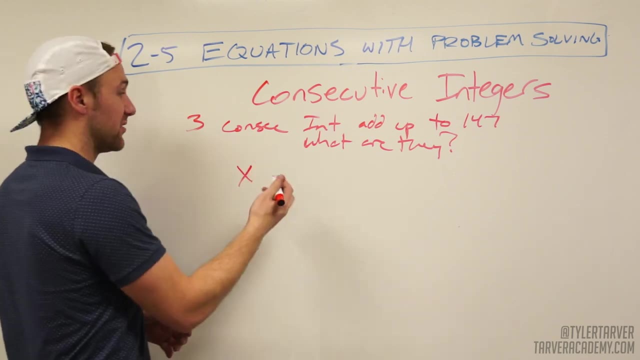 how it works. I didn't make the rules, So this is how you do the equation, All right. So I know that I've got three numbers. One of them is a number, and then they're consecutive. So I know that I've also got another number- That's just one more than that, And then I got another number. 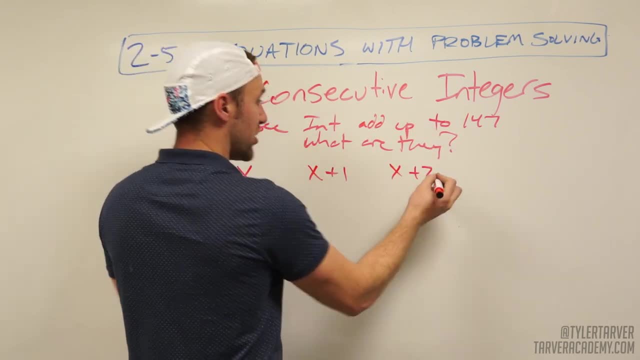 that I know is one more than that. So it'd be like this number plus two, correct? So I've got my original number. I know I went up one and then I went up two from there. So boom, boom, boom. 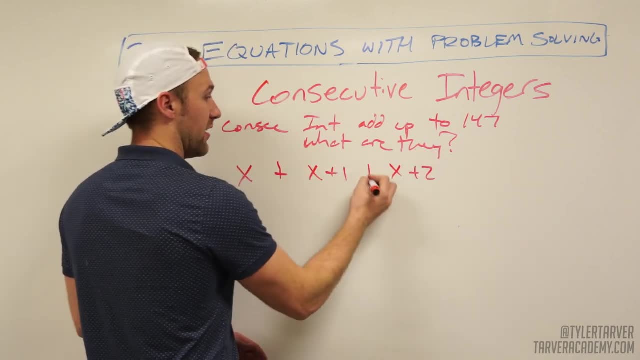 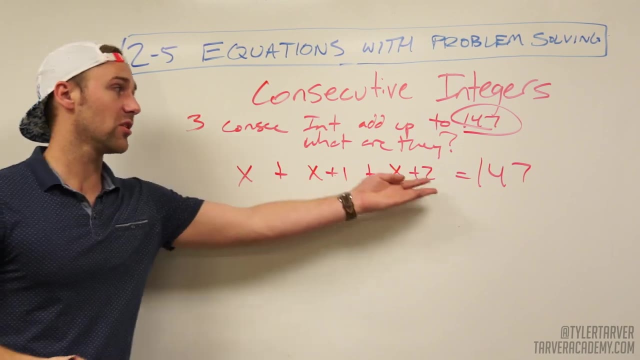 they're in a row. I know they add up. add up to equal 147.. All right, So now? oh, it looks so hard. No, it's not. Look dude, just split it at the equal sign and combine like: 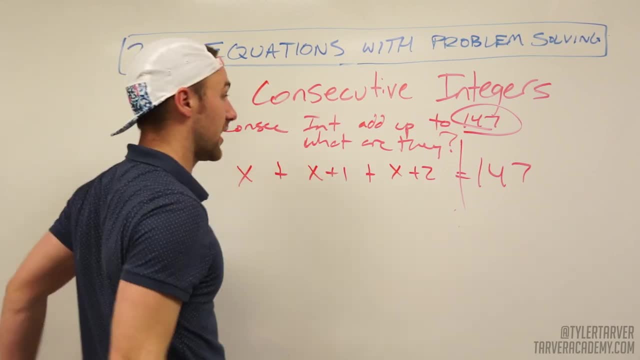 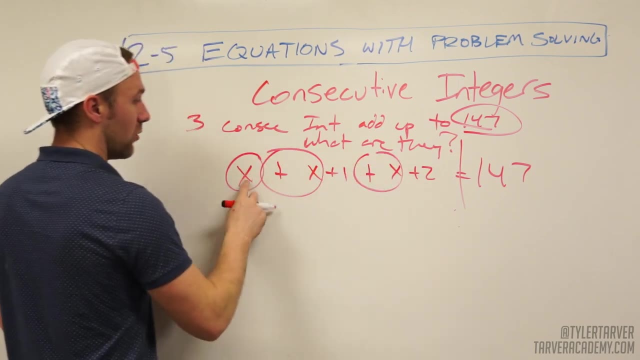 terms. Okay, You don't do any opposites unless you go across the equal sign. We're not going to go there yet. We're going to chill over here for a minute. So we've got X plus X plus X one- two. 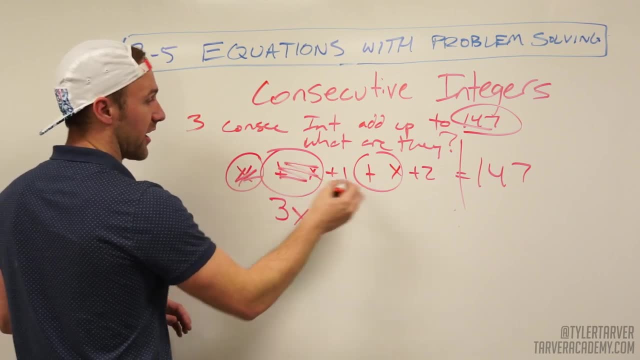 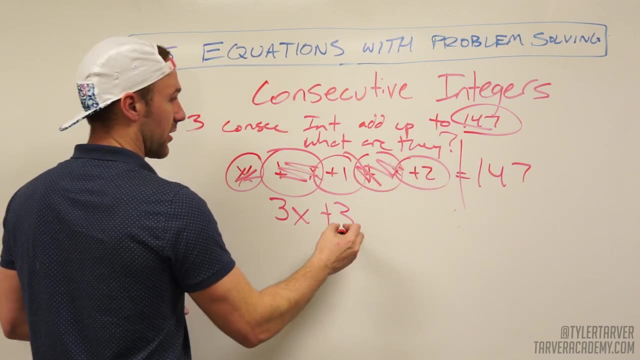 three, that's three X. I'm going to mark them out so I don't count them twice. I kept the signs with them. Now I'm going to do my regular numbers. One plus two is three. I'm going to bring down. 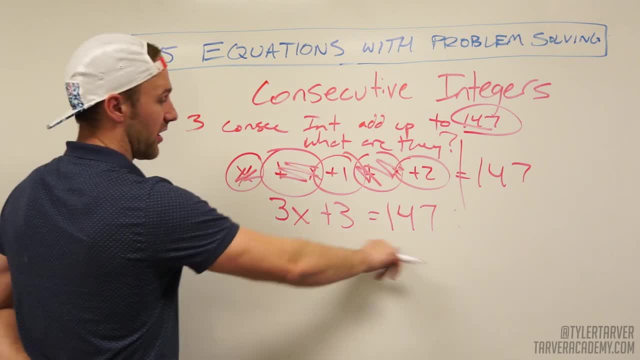 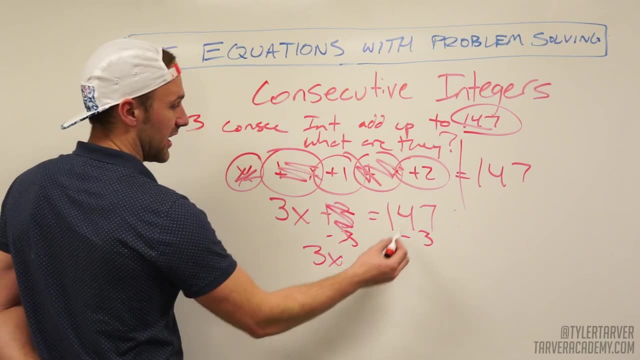 them. Now I'm going to go across the equal sign. I'm going to get rid of that one first because it's further away from the X. So minusing three, that cancels out Three X equals 144.. And I'm 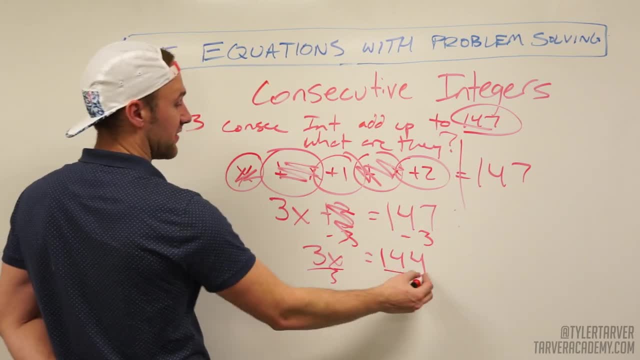 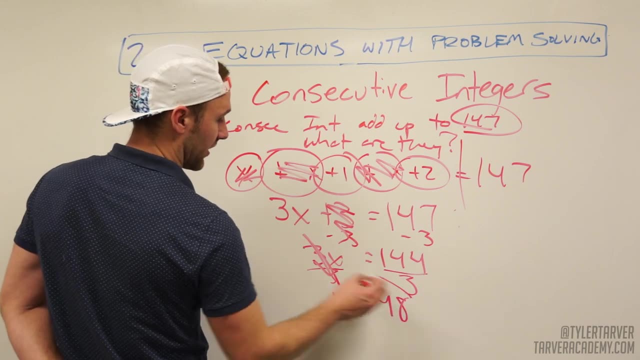 going to divide that by three, because three times X the opposite is divide. So we've got X, it cancels out, And then that goes into a four and then eight. So X equals 48. And you're like I'm done And that's going to be an answer. Well, don't do that, because they're probably